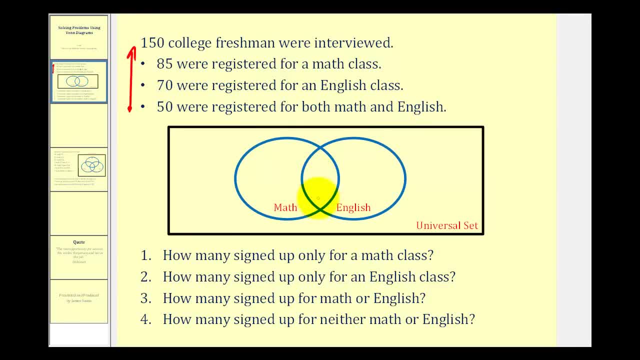 math and English. There are fifty students in this region, here where math and English overlap. Next, we're told that seventy were registered for an English class, And notice that of these seventy, fifty of them are also taking math. So seventy minus fifty leaves twenty students. 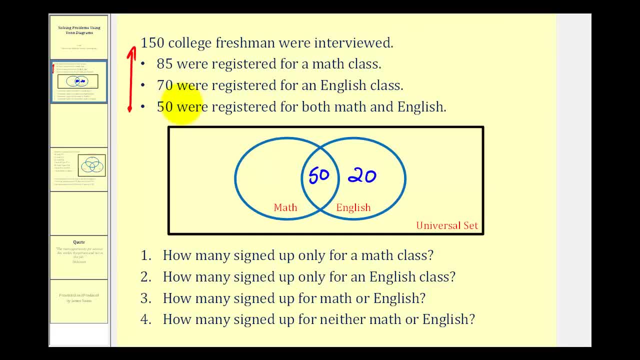 taking only English. So when it says seventy were registered for English, we have to also count those taking English and math, or these fifty here. And then eighty-five were registered for a math class. Again, fifty of the eighty-five are already accounted for, leaving thirty-five. that just 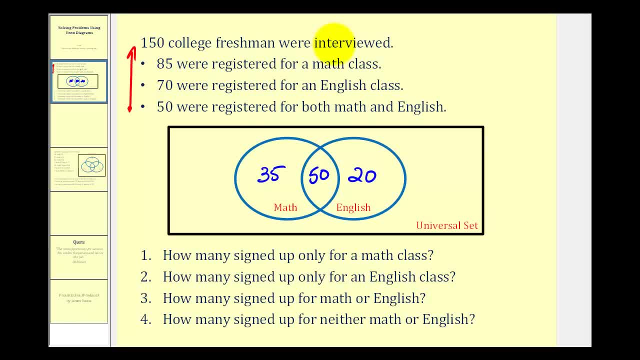 take math And since one hundred fifty students were interviewed, notice that thirty-five plus fifty plus twenty are the only students that have been accounted for so far, which is one hundred five students, Which means there must be forty-five students in this region here. 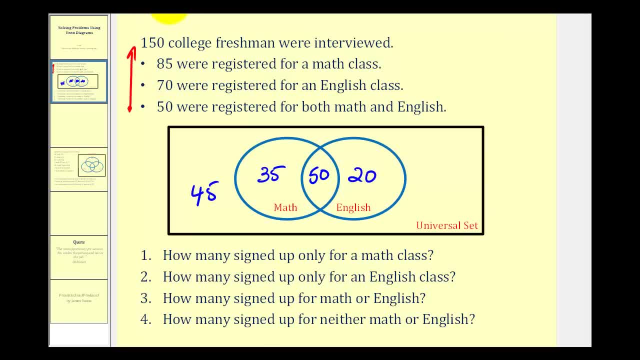 that are not taking math or English. Now let's answer the questions. Number one: how many signed up only for a math class? Well, that would be these thirty-five students here. How many signed up only for English class? That would be twenty. 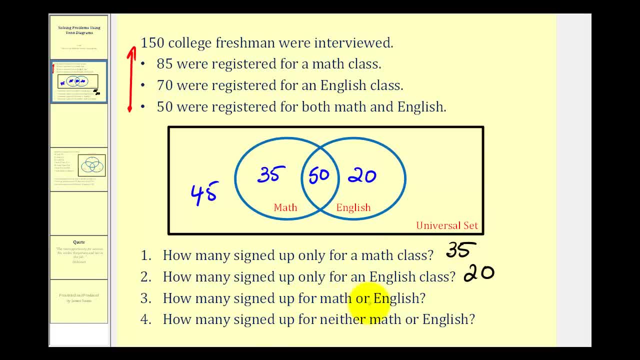 How many signed up for math or English? This question is asking for any student that took a math class or an English class, so it would be all the students in this entire region here. So thirty-five plus fifty, That's 85 plus 20, that's 105.. 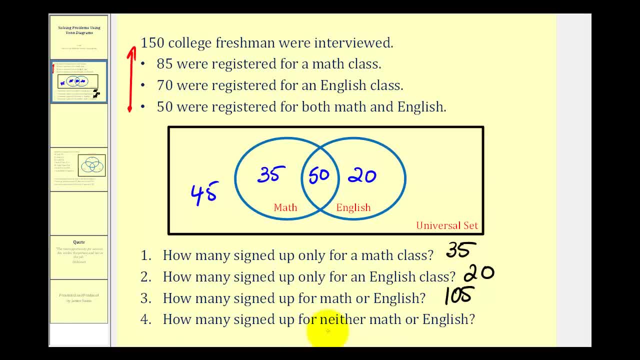 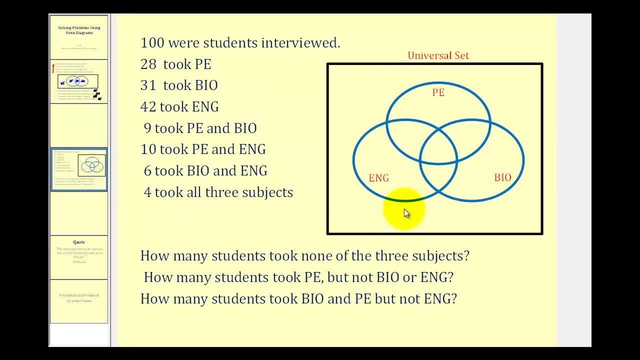 And then number four: how many signed up for neither math or English? That would be the students outside of our circles here, which would be 45 students. Now let's take a look at a second example And notice. for this one, we have three different courses to be considered. 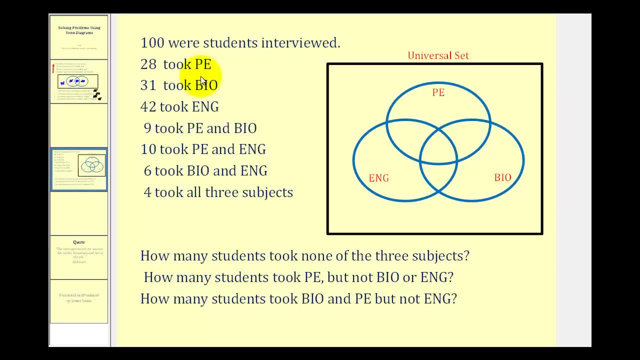 100 students were interviewed: 28 took PE, 31 took biology, 42 took English, 9 took PE and biology, 10 took PE and English, 6 took biology and English and 4 took all three subjects. Again, we're going to work our way from the bottom to the top. 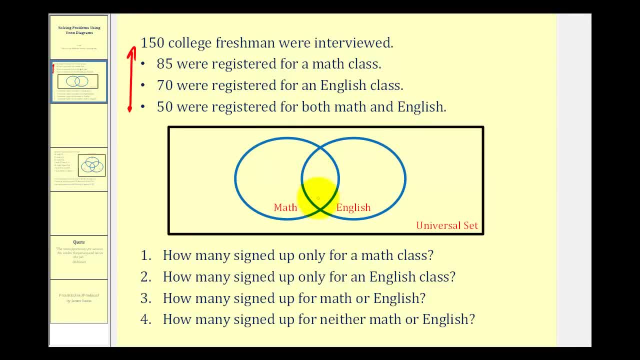 math and English. There are fifty students in this region, here where math and English overlap. Next, we're told that seventy were registered for an English class, And notice that of these seventy, fifty of them are also taking math. So seventy minus fifty leaves twenty students. 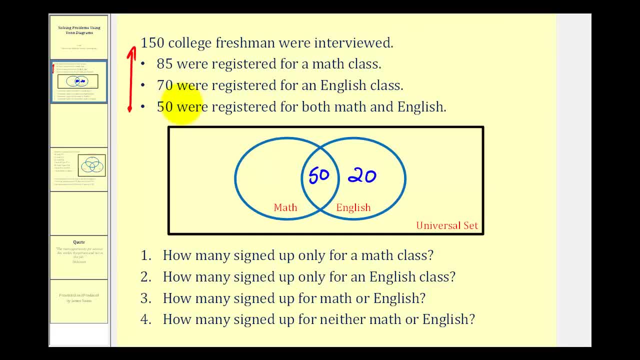 taking only English. So when it says seventy were registered for English, we have to also count those taking English and math, or these fifty here. And then eighty-five were registered for a math class. Again, fifty of the eighty-five were already accounted for, leaving thirty-five. that just 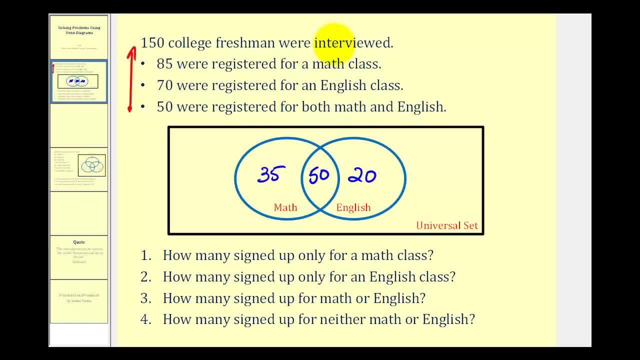 take math And since one hundred fifty students were interviewed, notice that thirty-five plus fifty plus twenty are the only students that have been accounted for so far, which is one hundred five students, Which means there must be forty-five students in this region here. 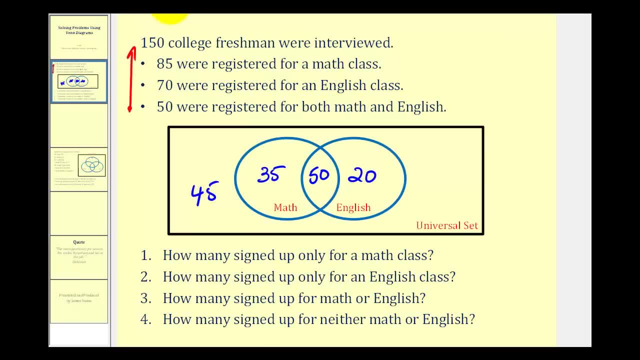 that are not taking math or English. Now let's answer the questions. Number one: how many signed up only for a math class? Well, that would be these thirty-five students here. How many signed up only for English class? That would be twenty. 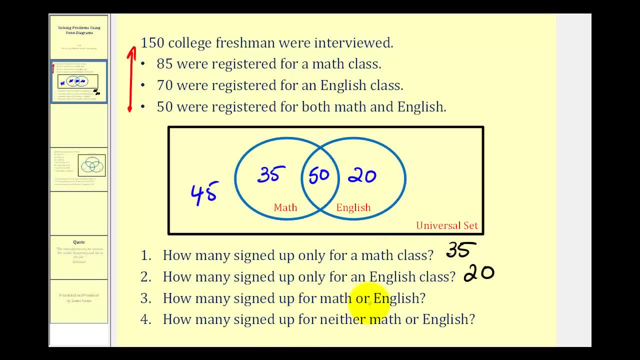 How many signed up for math or English? This question is asking for any student that took a math class or an English class, So it would be all the students in this entire region here. So thirty-five plus fifty, that's eighty-five Plus twenty, that's one hundred five. 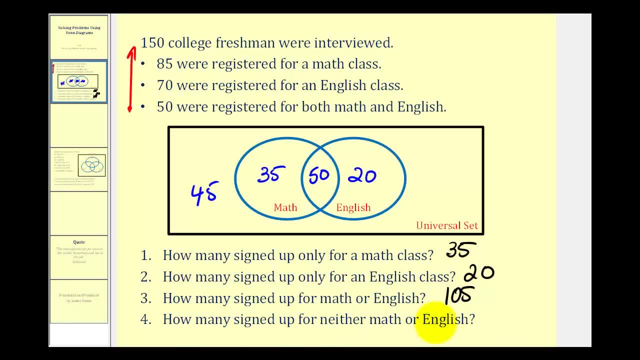 And then number four. how many signed up for neither math or English? That would be the students outside of our circles here, which would be forty-five students. Now let's take a look at a second example And notice. for this one we have three. 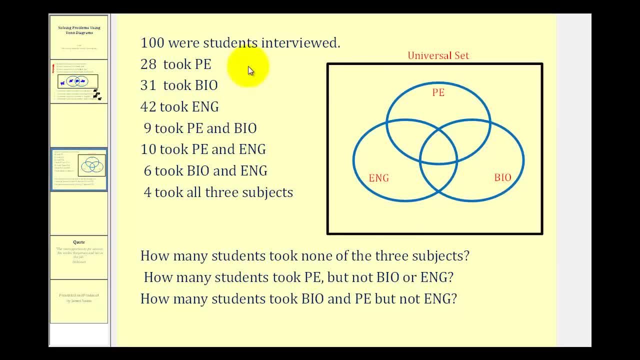 different courses to be considered. One hundred students were interviewed. Twenty-eight took PE, Thirty-one took biology, Forty-two took English, Nine took PE and biology, Ten took PE and English, Six took biology and English And four took 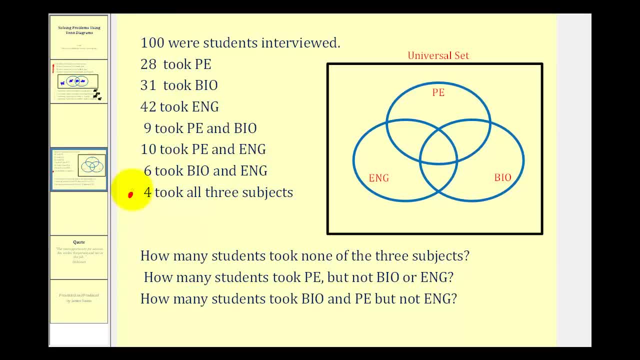 all three subjects. Again, we're going to work our way from the bottom to the top to complete our Venn diagram. So four students took all three subjects. The only region where all three subject overlap is in the middle here. So there are four students here. 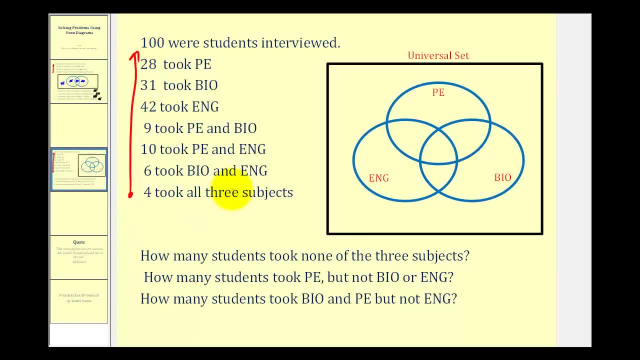 to complete our Venn diagram. So four students took all three subjects. The only region where all three subject overlap is in the middle here. so there are four students here. Next 6 took biology and English. Biology and English overlap in this region here. 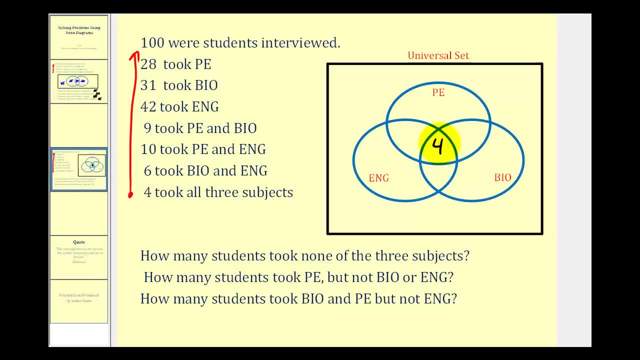 Notice that four of the six students are taking all three subjects. So that leaves only two students here that are taking only biology and English. So when it says 6 took biology and English, we also have to include the students that are taking all three subjects. 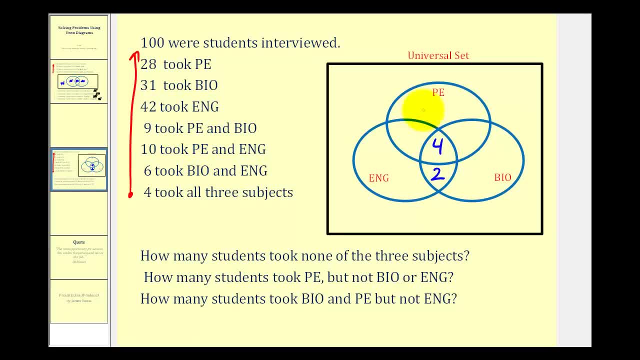 So if 10 took PE and English, that would be in this region here. Again, four of the 10 are in this region here, So we have 6 to make up a total of 10 taking PE and English, And then 9 took PE and biology. 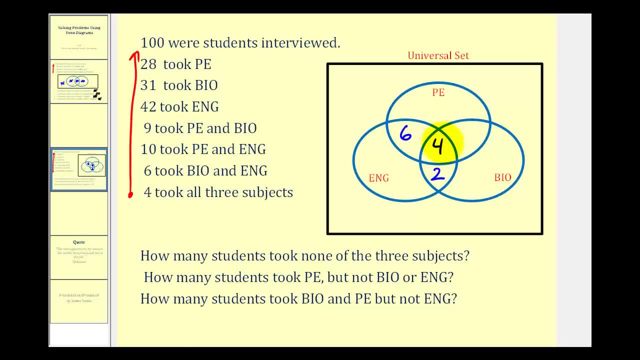 So for this region here, 4 of the 9 are already accounted for, leaving 5 in this region here that are taking only PE and biology. Again notice: 9 total are taking PE and English. as stated, 42 took English. So the number of students in this entire region here must be 42. 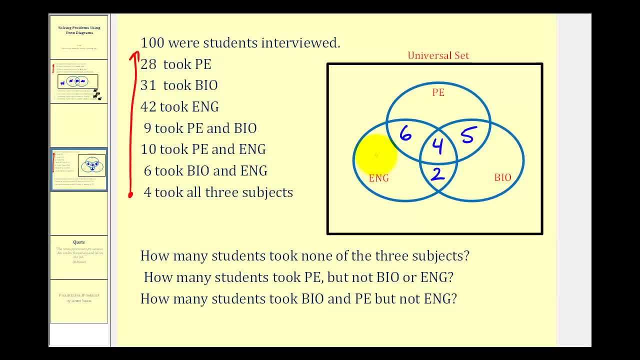 Again notice that 12 have already been accounted for, leaving 30 that take only English And then 31 took biology. Well, again notice that this region here is biology. 5 plus 4 plus 2 or 11 students are already accounted for. 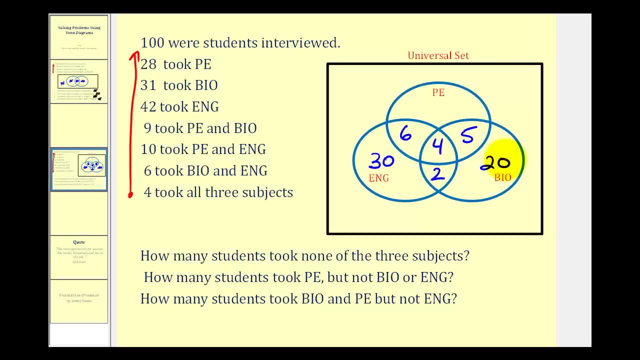 leaving 20 in this region here, And then we have 28 took PE. Notice that 15 are already accounted for. that take PE, leaving 13 in this region here, And these 13 only take PE. Now, the last step is to determine of these 100 students. 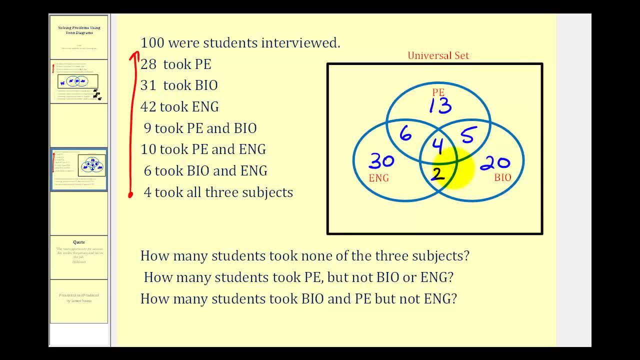 how many are not taking any of these three subjects. So let's see how many students have been accounted for. We have 30 plus 20 plus 13.. That's 63.. Plus 6 plus 4 plus 5 plus 2.. 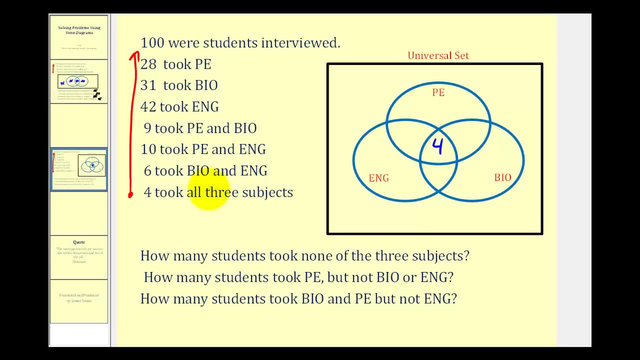 Next, six took biology and English. Biology and English overlap in this region here. Notice that four of the six students are taking all three subjects. So that leaves only two students here that are taking only biology and English. So when it says six took biology and English, 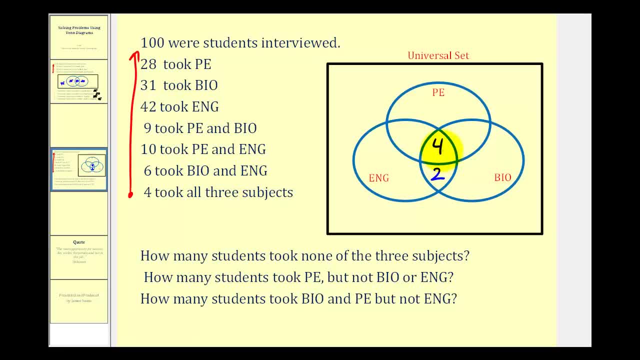 we also have to include the students that are taking all three subjects. So if ten took PE and English, that would be in this region. here Again, four of the ten are in this region, So we have six to make up a total of ten taking. 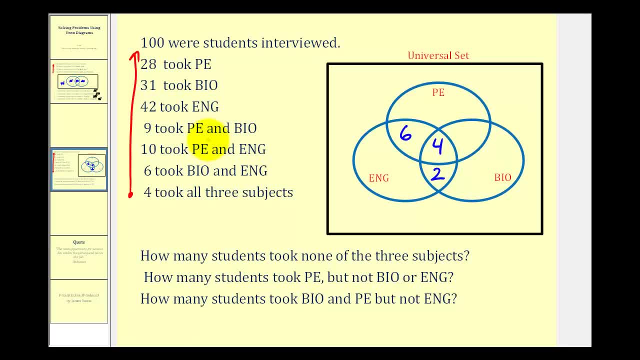 PE and English. And then nine took PE and biology. So for this region here four of the nine are already accounted for leaving five in this region here that are taking only PE and biology. Again notice: nine total are taking PE and English. 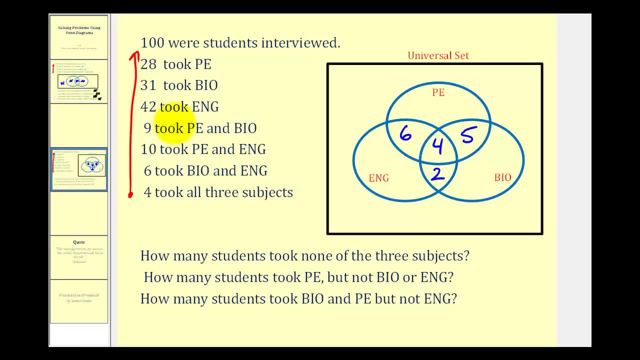 as stated, Forty-two took English, So the number of students in this entire region here must be forty-two. Again, notice that twelve have already been accounted for, leaving thirty that take only English. And then thirty-one took biology. Well, again, notice that this region here is biology. 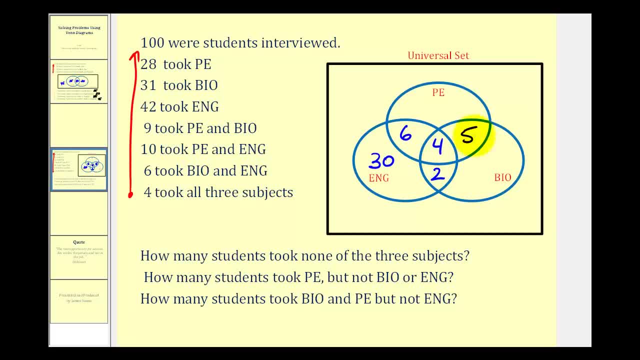 Five plus four plus two or eleven students are already accounted for, leaving twenty in this region here, And then we have twenty-eight. took PE. Notice that fifteen are already accounted for. that take PE, leaving thirteen in this region here, And these thirteen only take PE. 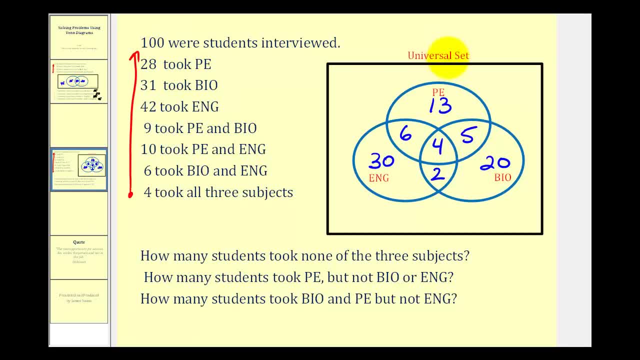 Now the last step is to determine, of these one hundred students, how many are not taking any of these three subjects. So let's see how many students have been accounted for. We have thirty plus twenty plus thirteen, that's sixty-three plus six plus four plus five plus two. 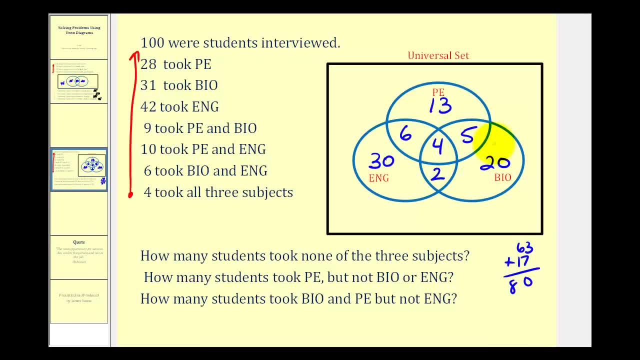 that's seventeen. So eighty students have been accounted for of the one hundred, leaving twenty more that are not taking any of these three subjects. Now that we have the Venn diagram completed, we should be able to answer all these questions. How many students took none of the three subjects? Well, that would be twenty.